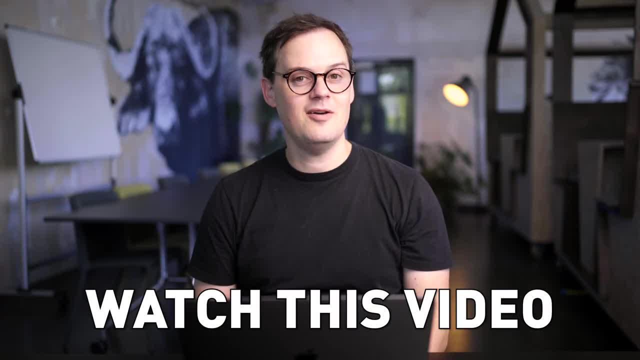 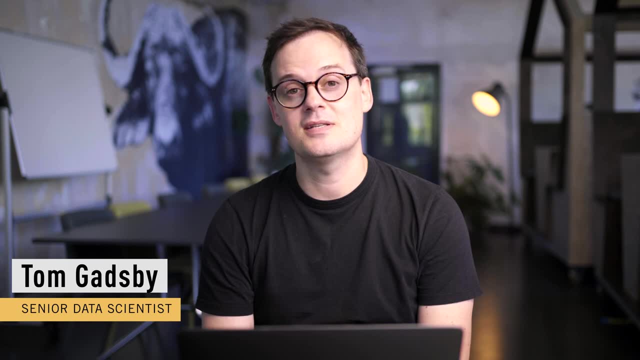 Have you read articles about how cool it is to be a data analyst? Watch this video and find out if it suits you. My name's Tom. I've been working in the field for more than five years and I'm currently a senior data scientist at Career Foundry. Data analyst is one of the hottest job. 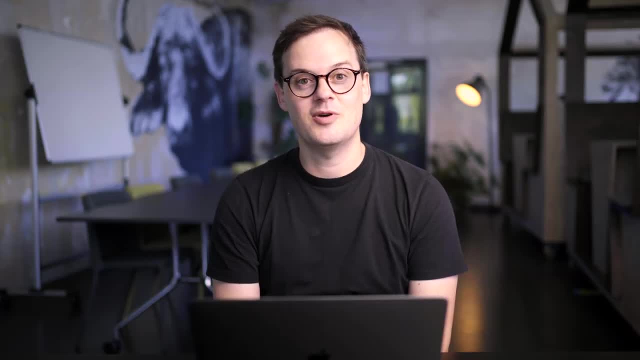 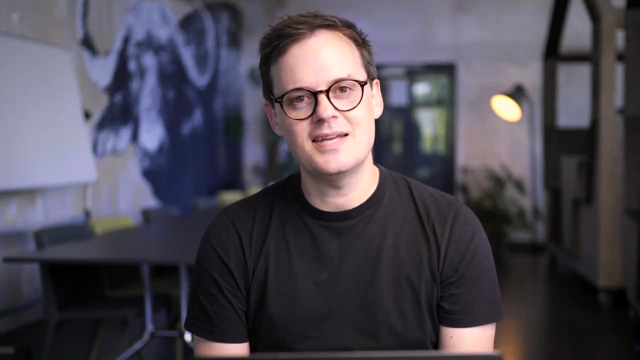 titles in 2022.. A job in data promises exciting career prospects, so it's no surprise that more and more people are transitioning into the field, and with the demand comes great salaries. So what does it take to thrive in this industry and how do you know if it's the right career for you? Career. 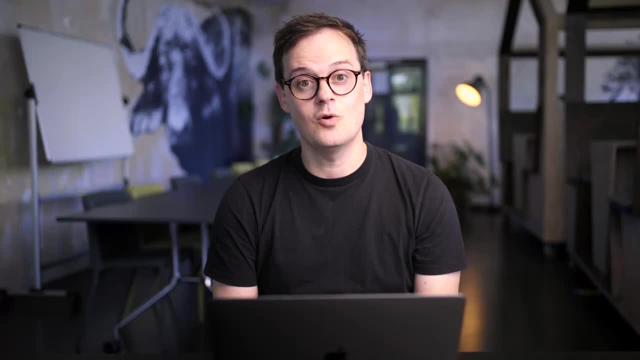 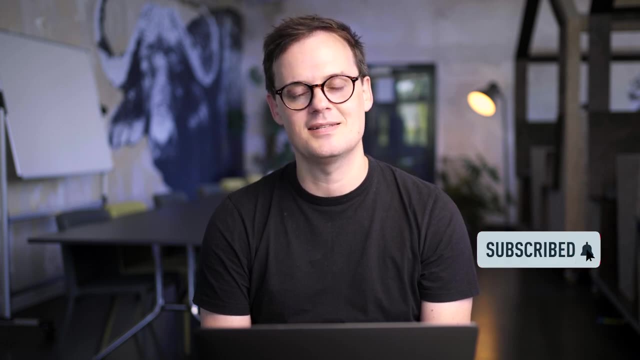 change isn't easy, and it's not just about salary and job title. You also have to love what you're going to do and be good at it. So in this video, we'll help you figure out if you have what it takes to be a good data analyst and, more importantly, whether a career in data analytics 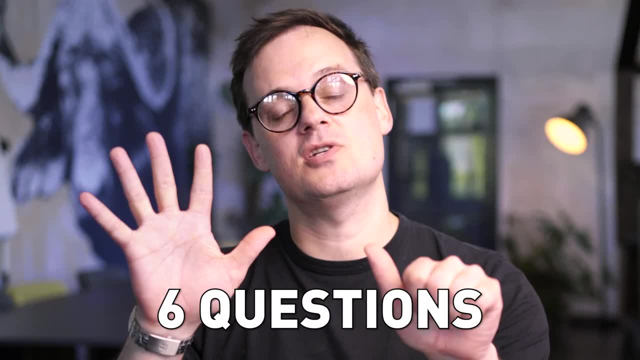 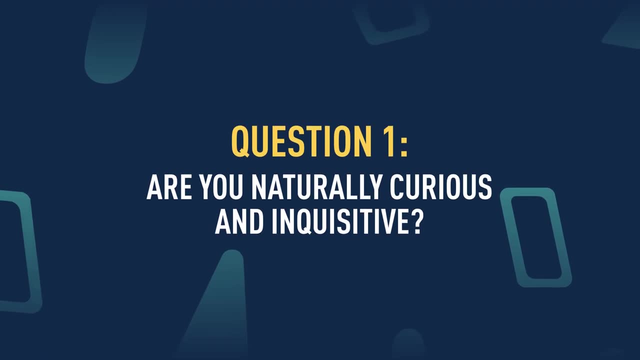 aligns with your own goals and objectives? Here are six questions you'll need to ask yourself before starting a career in data analytics. So let's start with question number one. Are you naturally curious and inquisitive? Analytics is about trying to find insights from data. 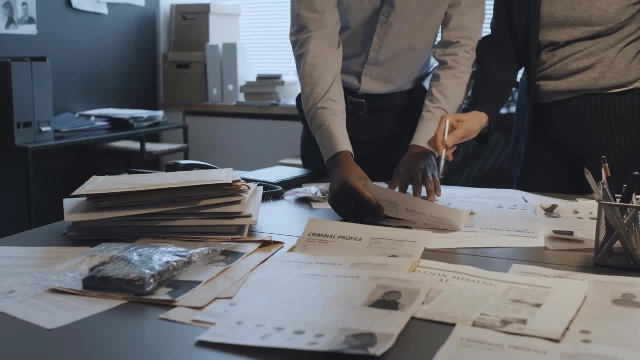 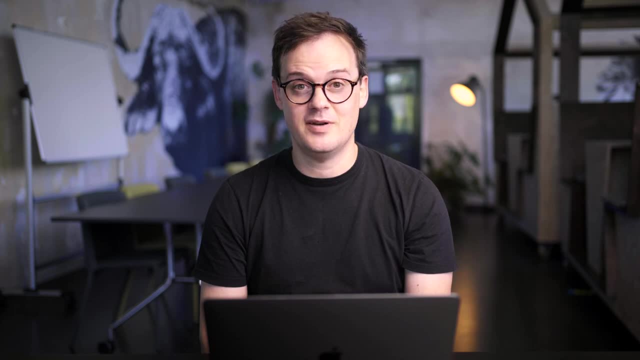 Think of yourself like a data detective. And just like detectives, clues in the data are often hidden where other people haven't thought to look. You will need to work hard and dig deep into the data to find insights. This means you'll be operating in uncertainty A lot of the time. you'll be working by yourself. Are you comfortable? 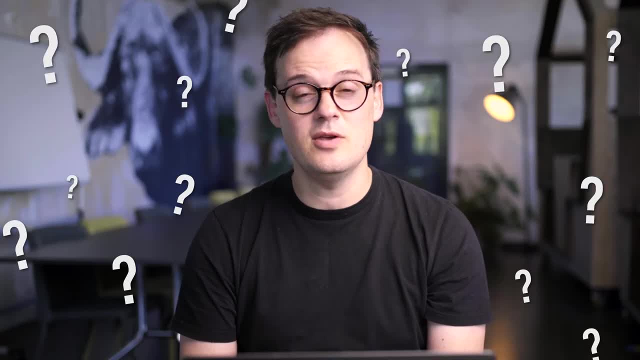 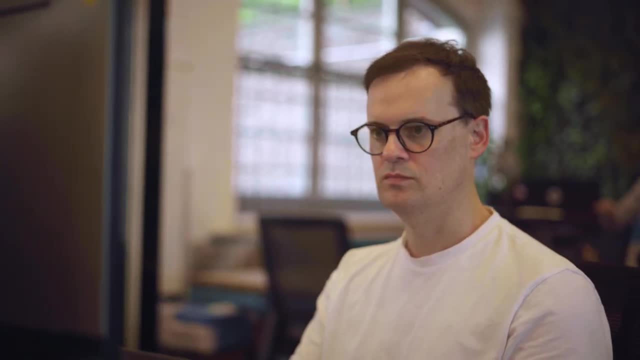 working in uncertainty and admitting to yourself you don't really know where you need to go. You will also make a lot of mistakes. Finding new insights involves trial and error. Are you confident in your ability to solve something despite having failed at it four or five times previously? Check? 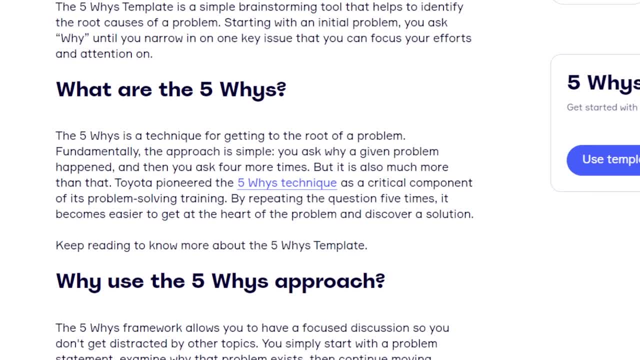 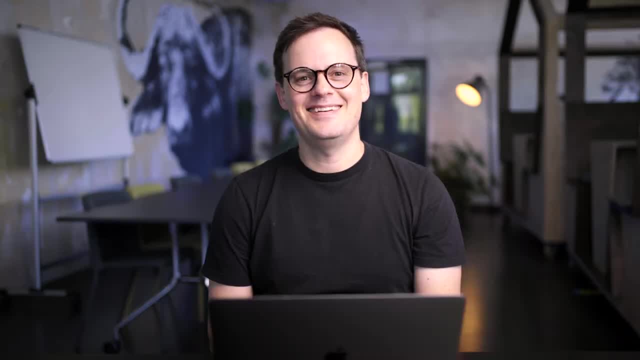 your data analytics skills. Do you have a good data analysis technique or root cause analysis? These are techniques that help you develop a rigorous problem-solving mindset. You might find you already have them, in which case you're naturally a good fit for data analytics Now. 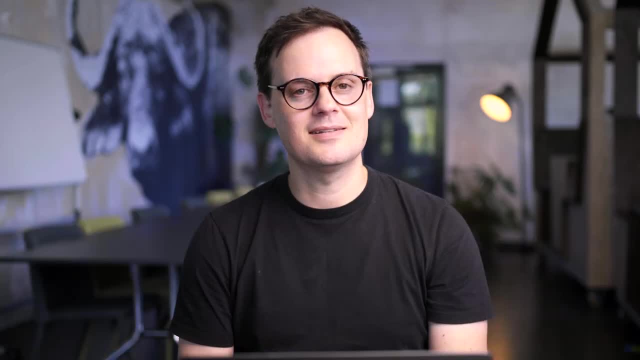 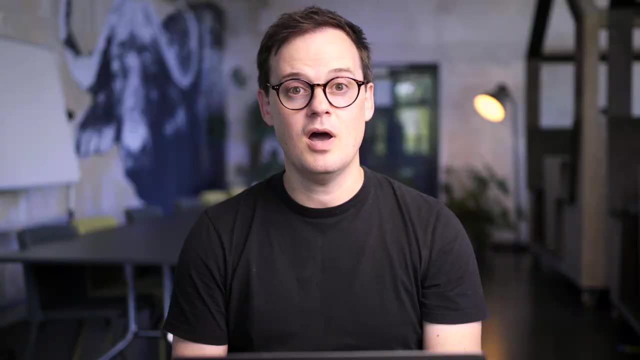 onto question number two: Do you have an analytical mindset and a logical approach to your work? Good data analysts have an analytical mindset. They make data-driven decisions. They have learned that data-driven insights are not easily discovered, Relying solely on intuition and inspiration. can 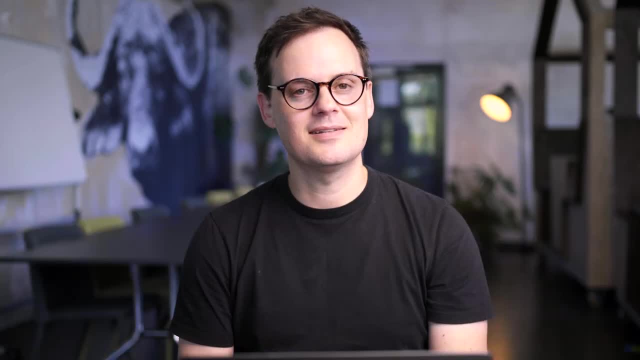 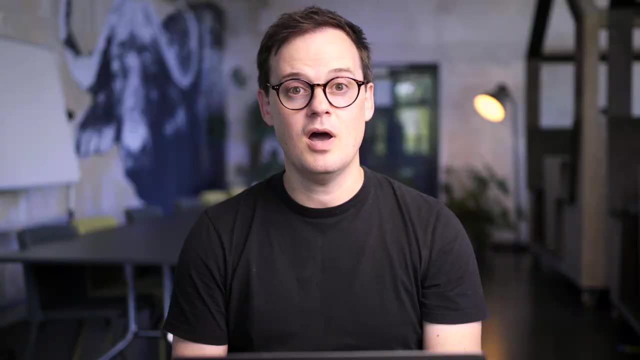 onto question number two: Do you have an analytical mindset and a logical approach to your work? Good data analysts have an analytical mindset. They make data-driven decisions. They have learned that data-driven insights are not easily discovered, Relying solely on intuition and inspiration. can 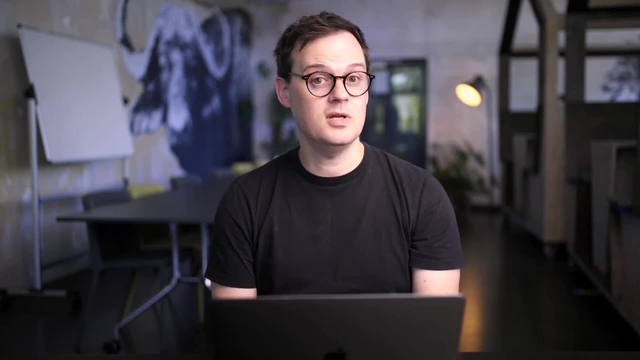 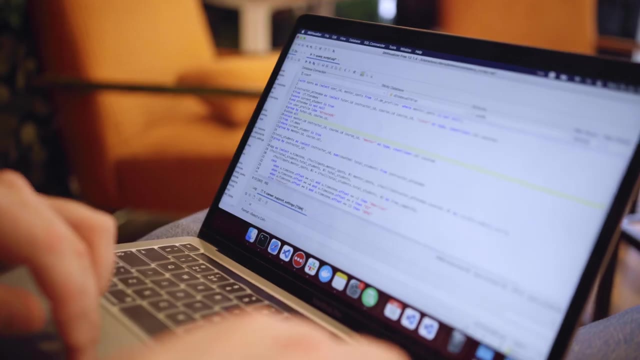 often fail. on complex problems, Truths can be discovered by combining human intuition with the power of our computational cousins. Effective data analysts build logical processes that rely on insights derived from data. Do you tend to work methodically, from A to Z, questioning everything? 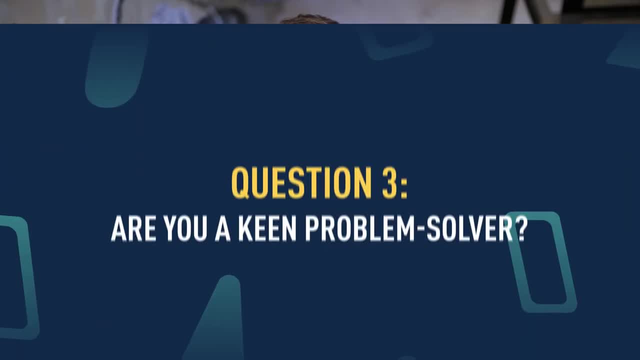 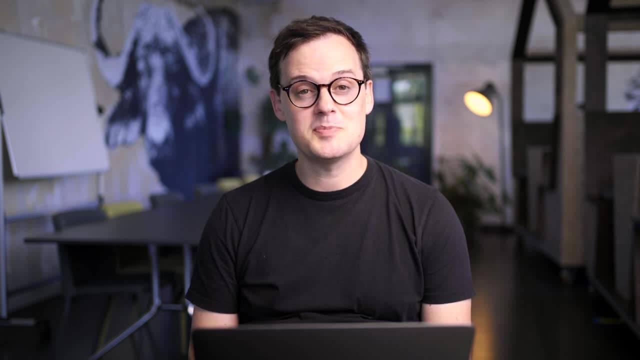 rather than making assumptions, Amazing. Onto question number three: Are you a keen problem solver? Data analytics is the process of rigorous problem solving. Good data analysts are curious people who like to problem solve. Do you like puzzles? Are you inspired when you learn something? 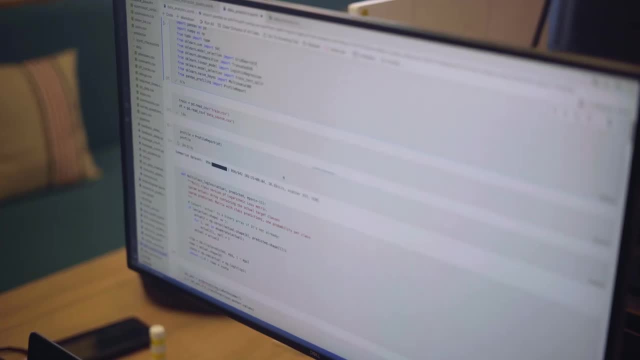 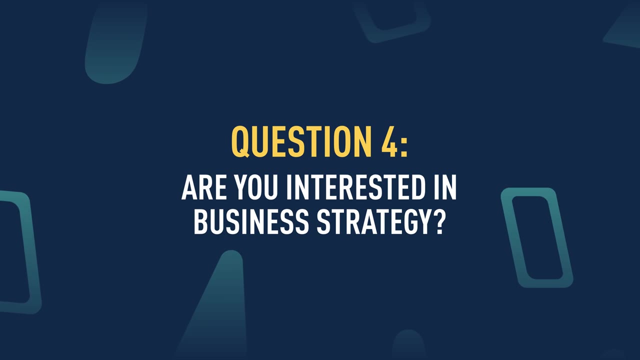 new. Also, if you don't have the necessary data to hand, you may need to go and find it, which in and of itself is a problem-solving exercise. Question number four: Are you interested in business strategy? Let's be honest, You can do data analytics on any problem you find interesting, In fact. 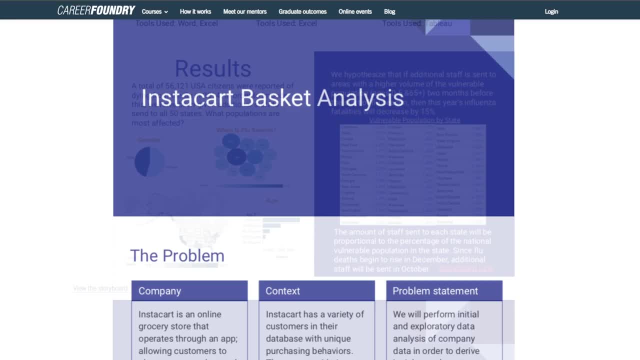 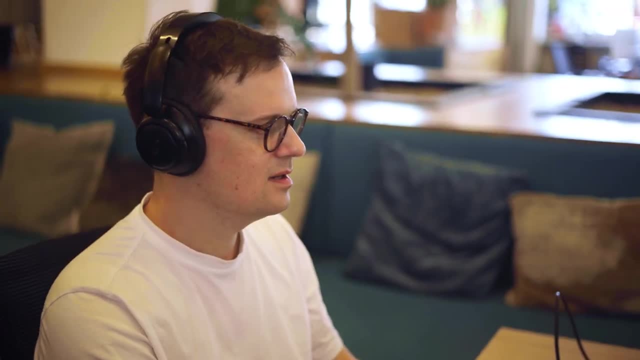 this is one of the best ways for you to learn about the field, build up a portfolio and land your first job in data analytics. But in reality, you'll spend most of your career working for a business. You'll need to bridge the gap between the numbers and the real-world implications. 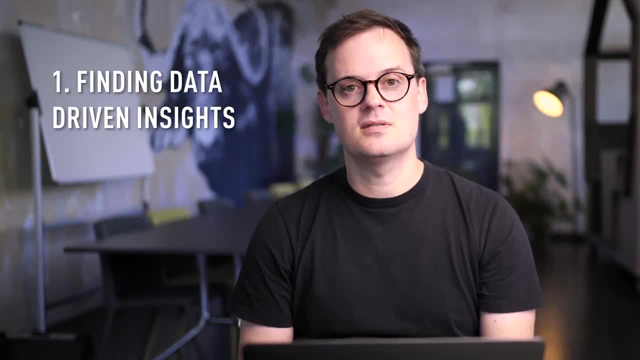 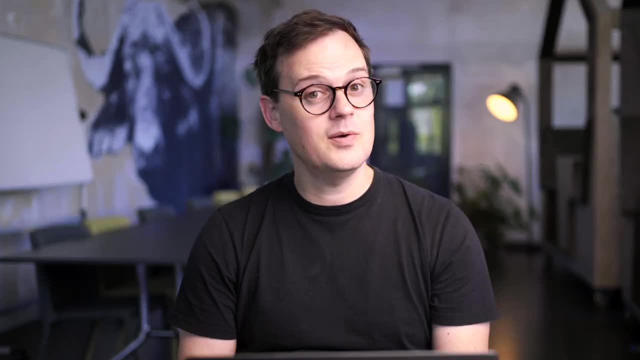 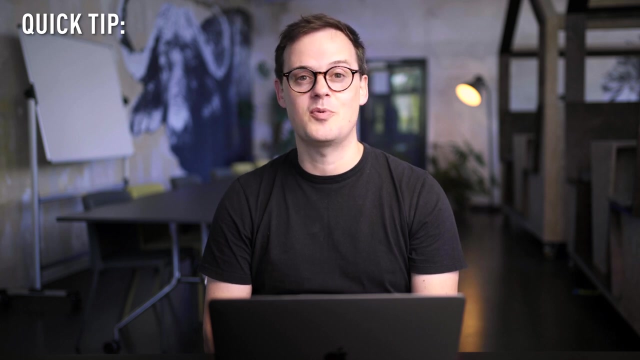 for the business. So finding data-driven insights and helping the business drive its strategy through data-driven decisions will be some of your primary responsibilities. Are you interested in driving business strategy? Quick tip: It also helps if you're interested in the sector or geography that the business operates in. 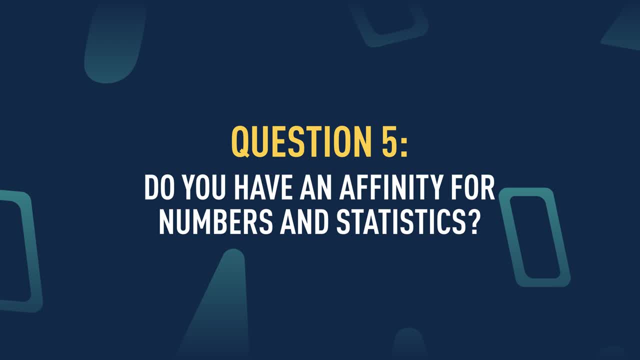 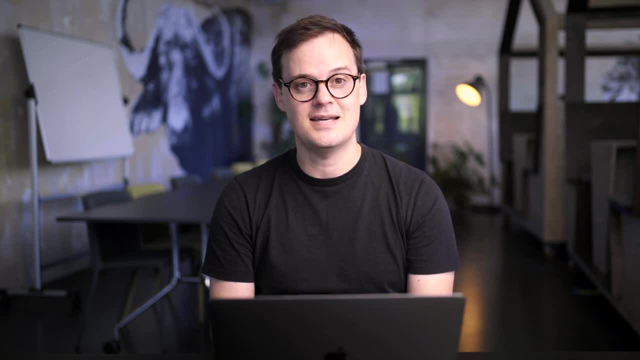 Moving on to question number five, Do you have an affinity for numbers and statistics? Well, this doesn't need to be a scary one. You don't need to be a maths genius to excel in data analytics. In fact, you do. You don't even need a maths background. You can learn everything you need during training. 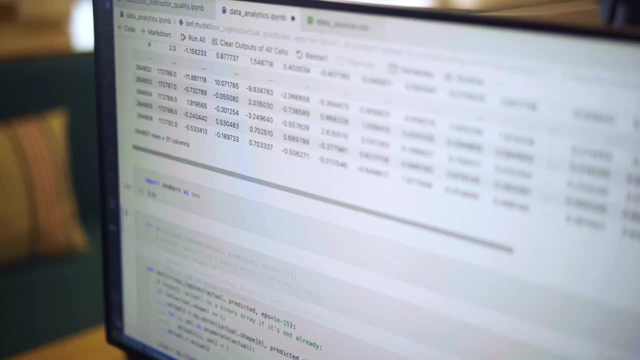 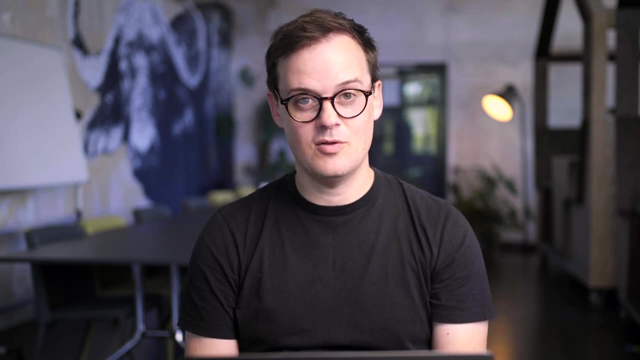 You do need to be comfortable working with numbers, in particular statistics. It's going to form a large part of your job. Do you break out in a cold sweat when given an Excel spreadsheet, Or are you happy to think about the real world through the lens of numbers? 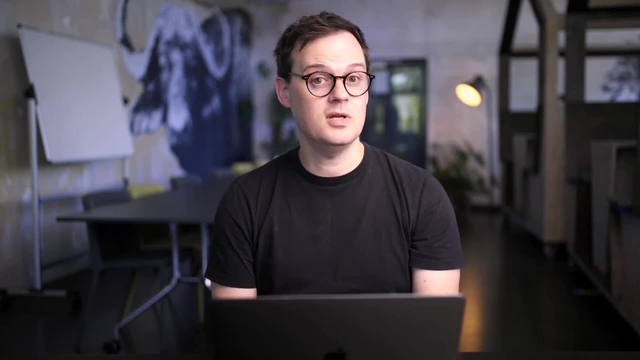 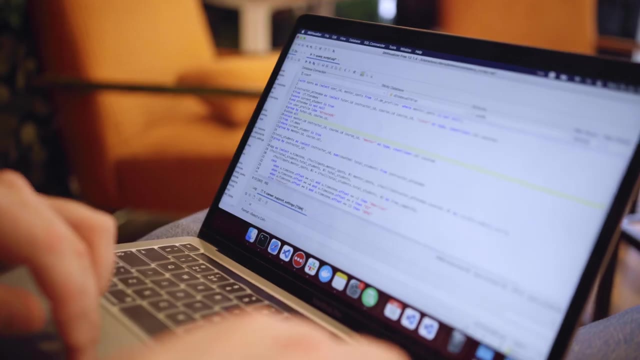 often fail. on complex problems, Truths can be discovered by combining human intuition with the power of our computational cousins. Effective data analysts build logical processes that rely on insights derived from data. Do you tend to work methodically, from A to Z, questioning everything? 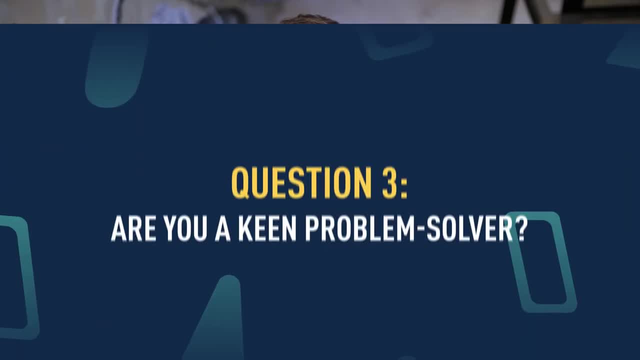 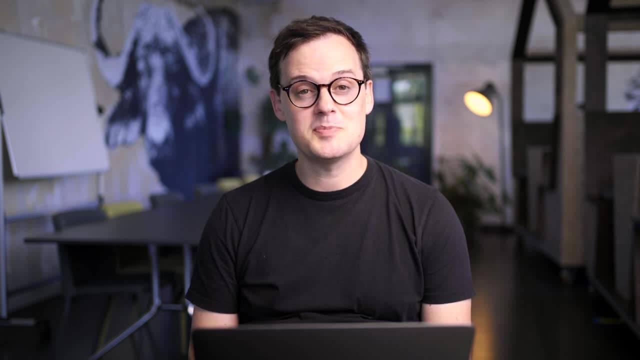 rather than making assumptions, Amazing. Onto question number three: Are you a keen problem solver? Data analytics is the process of rigorous problem solving. Good data analysts are curious people who like to problem solve. Do you like puzzles? Are you inspired when you learn something? 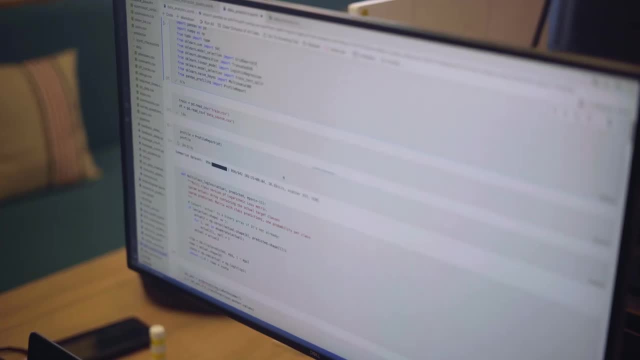 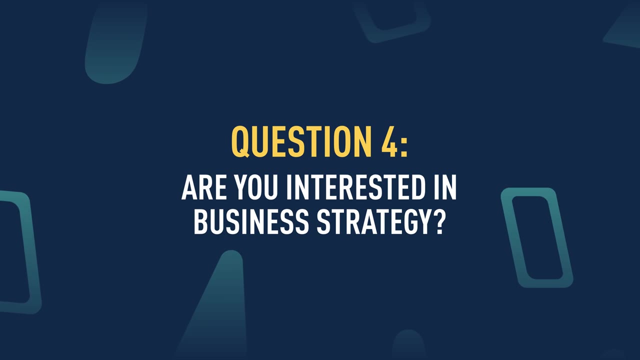 new. Also, if you don't have the necessary data to hand, you may need to go and find it, which in and of itself is a problem-solving exercise. Question number four: Are you interested in business strategy? Let's be honest, You can do data analytics on any problem you find interesting, In fact. 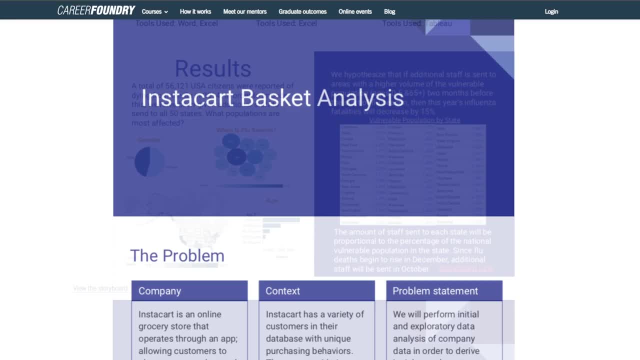 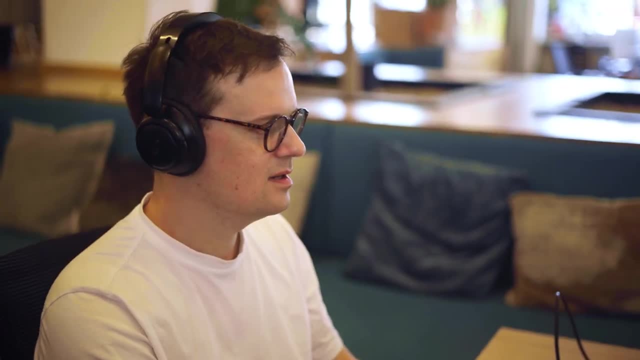 this is one of the best ways for you to learn about the field, build up a portfolio and land your first job in data analytics. But in reality, you'll spend most of your career working for a business. You'll need to bridge the gap between the numbers and the real-world implications. 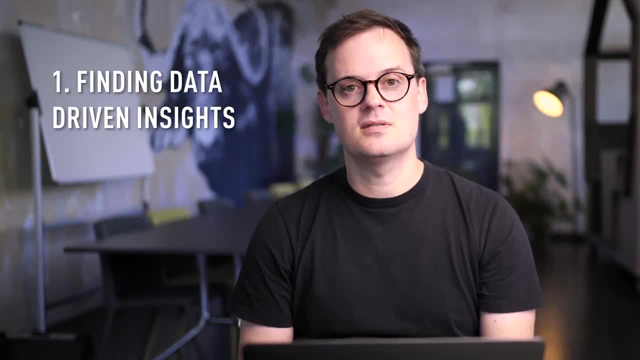 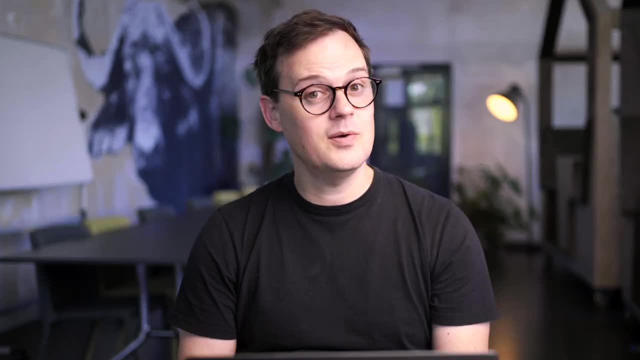 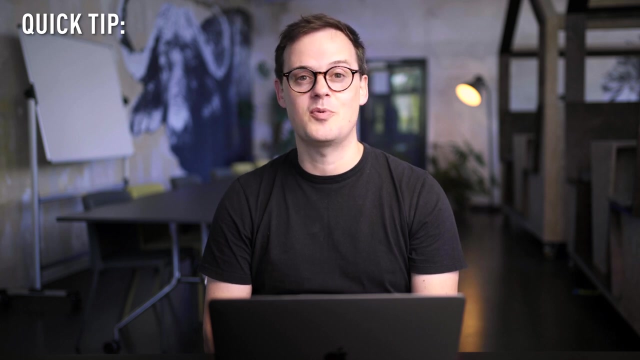 for the business. So finding data-driven insights and helping the business drive its strategy through data-driven decisions will be some of your primary responsibilities. Are you interested in driving business strategy? Quick tip: It also helps if you're interested in the sector or geography that the business operates in. 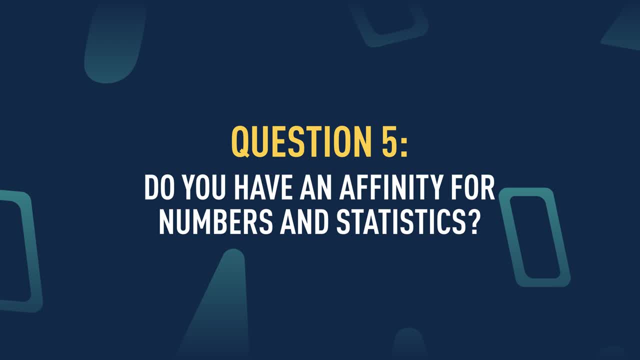 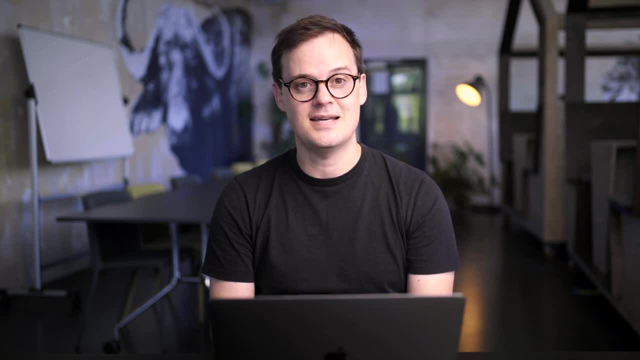 Moving on to question number five, Do you have an affinity for numbers and statistics? Well, this doesn't need to be a scary one. You don't need to be a maths genius to excel in data analytics. In fact, you do. You don't even need a maths background. You can learn everything you need during training. 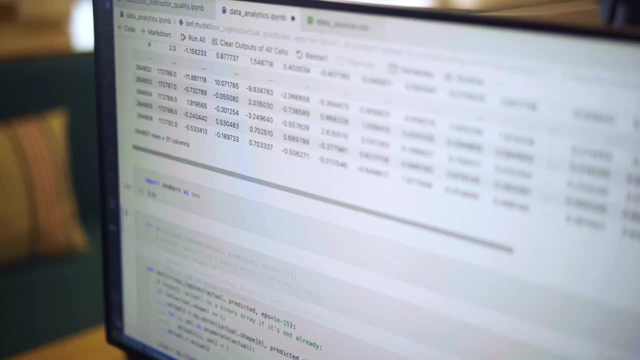 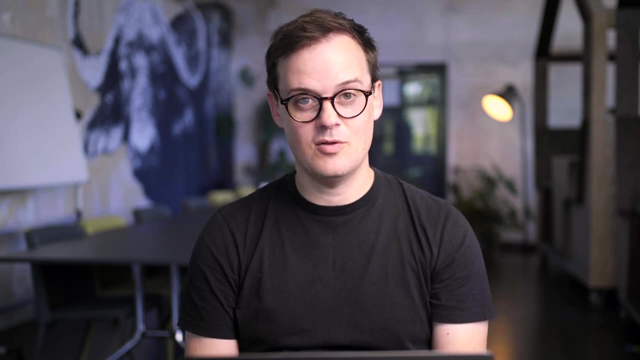 You do need to be comfortable working with numbers, in particular statistics. It's going to form a large part of your job. Do you break out in a cold sweat when given an Excel spreadsheet, Or are you happy to think about the real world through the lens of numbers? 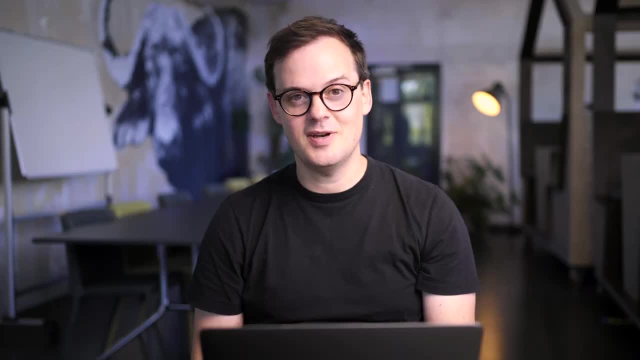 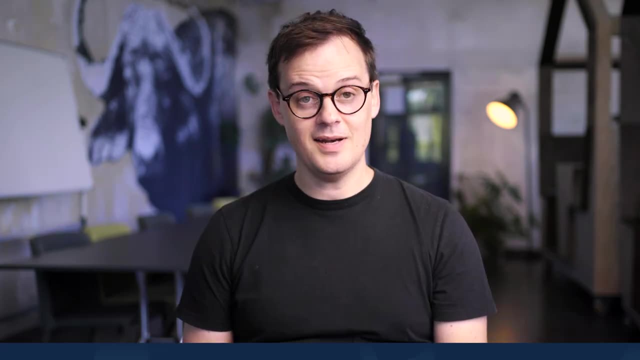 If so good. If you're finding this video helpful, please like this video and subscribe to the Career Foundry channel to keep up to date with all the data analytics content coming in the next few weeks. And finally, question number six: Are you comfortable presenting a? 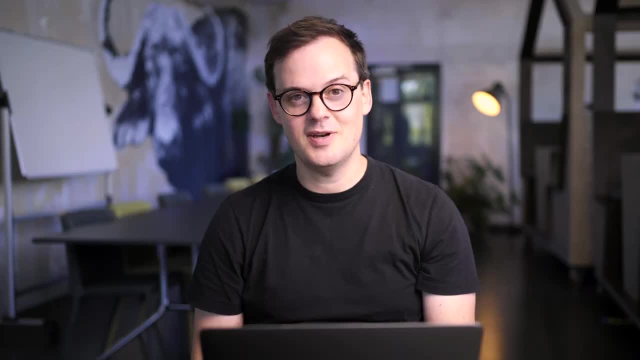 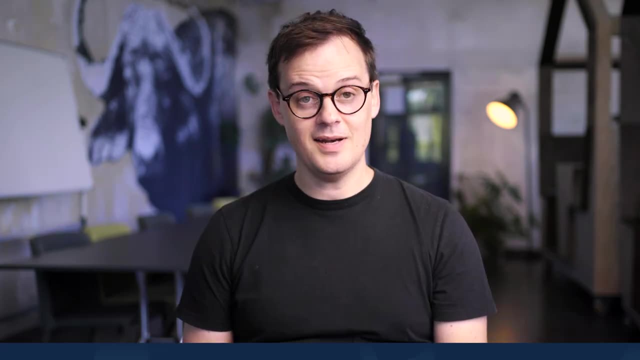 If so good. If you're finding this video helpful, please like this video and subscribe to the Career Foundry channel to keep up to date with all the data analytics content coming in the next few weeks. And finally, question number six: Are you comfortable presenting a? 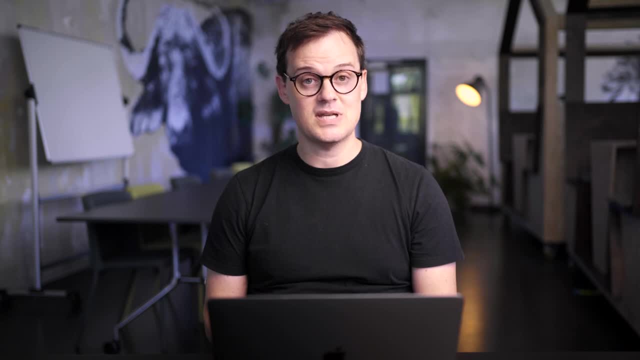 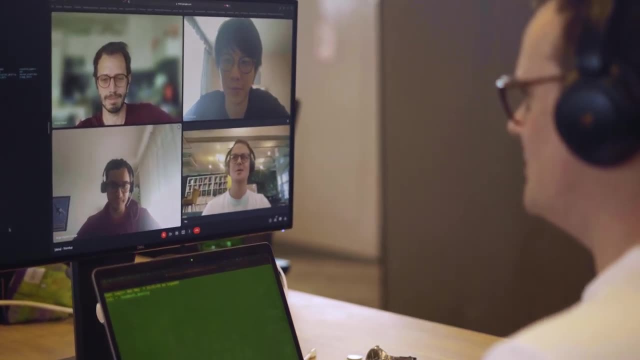 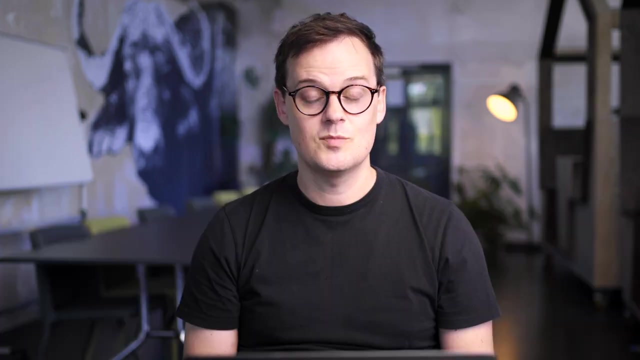 story and collaborating. Best data analysts are storytellers. They can present complex findings in a way non-data experts can understand. So do you have a knack for explaining tricky concepts in a clear and concise manner? Also, data analysts need to help the business take action derived from the data. 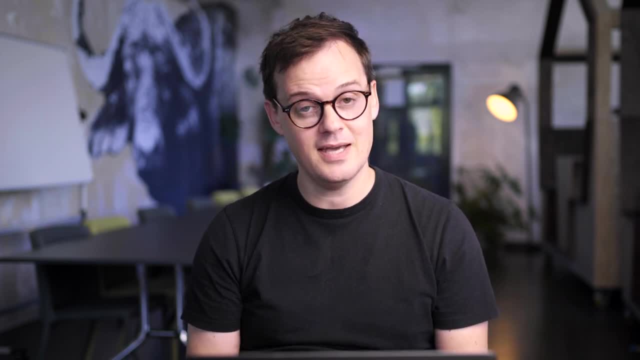 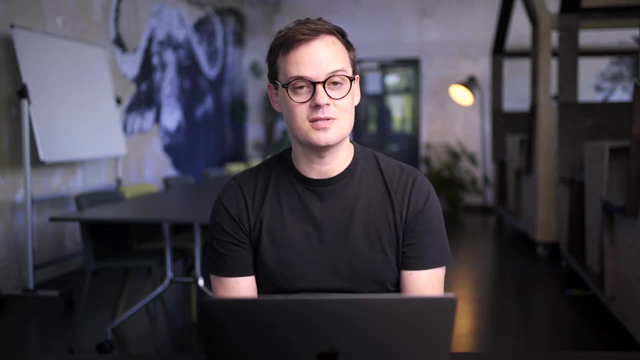 So are you a confident presenter and happy to argue your case? These qualities will serve you well in the role of data analyst. Now we've given you the questions to ask yourself. we will answer one of the questions and answer the rest of the questions in the Q&A section of the Q&A section of the Q&A section. So let's start with the first question. What is a good career move for a data analyst, And here are some reasons why: A competitive salary Based on data submitted by over 5,000 data analysts. the average base salary for a data analyst in the United States is around $75,000.. So a career as a data analyst could see you earning well above average salaries. Not only that, data analysts can expect strong salary growth as they gain more experience in the job market. A large factor in this has to do with the lack of highly experienced data analysts in the job market. 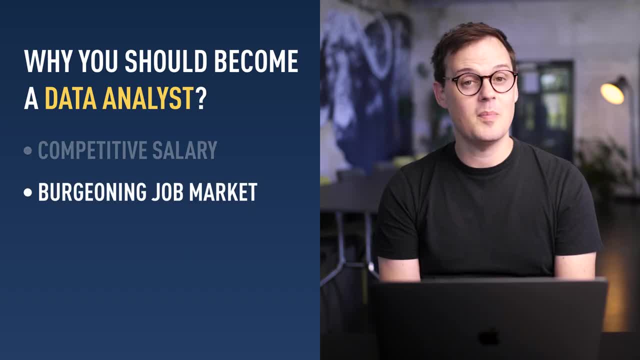 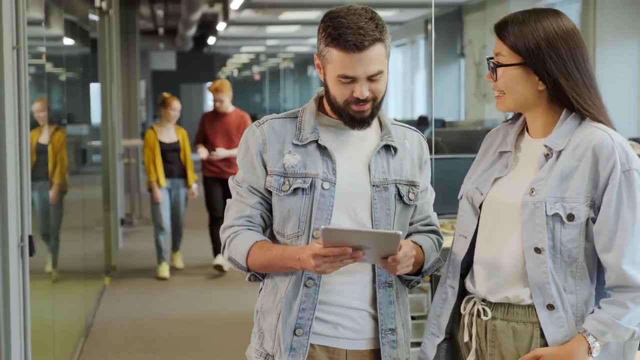 And this brings us on to the next point: a burgeoning job market. So, as we've already mentioned, there is an increasing demand for talented data analysts. More and more business sectors are transitioning towards a digital-first approach And, with the rise of connected devices and smartphone usage, 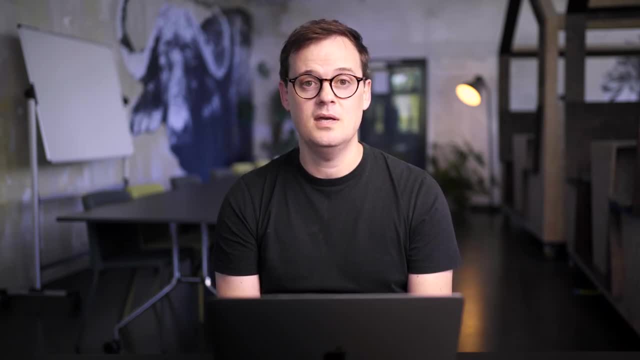 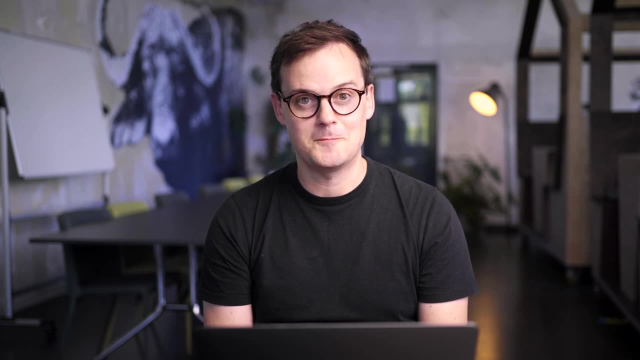 et cetera. the amount of data being generated by the modern economy is growing almost exponentially. Associated with this growth is an increasing need for data literate people in the job market. But supply is not meeting demand. Data isn't going anywhere, and neither are data analysts. 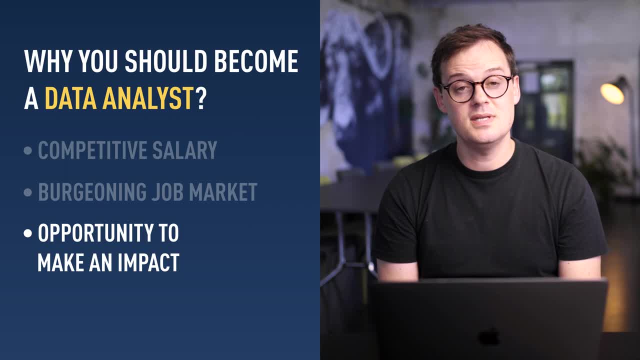 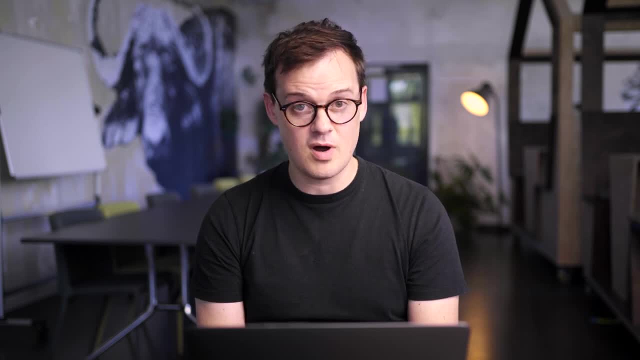 So this is an excellent job market to be a part of The opportunity to make an impact. Analytics plays a crucial role in how decisions are made. As a data analyst, you have an opportunity to drive business strategy and have a real impact on how the business moves forward. 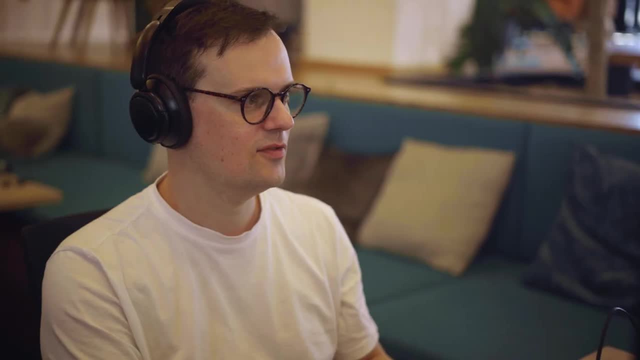 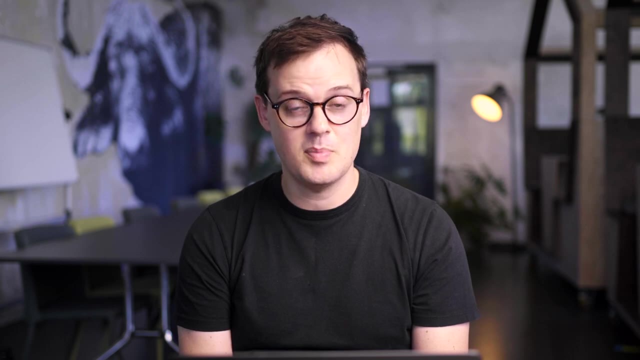 You'll get to the heart of complex business challenges, working closely with key stakeholders and using your expertise to advise on the best course of action. In this respect, you'll have a direct hand to play in the company's success and extremely rewarding. 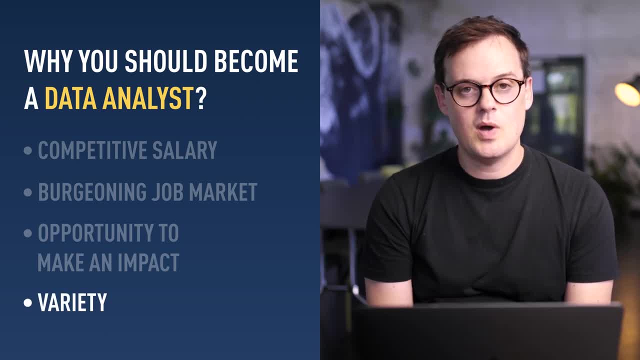 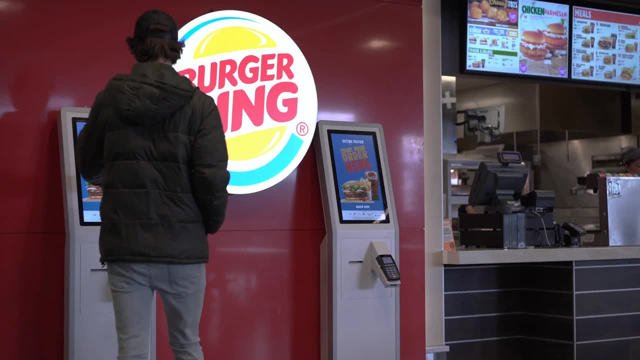 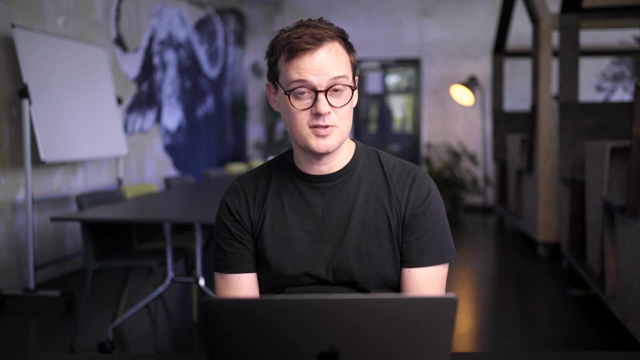 Variety. Data is absolutely everywhere, and there are opportunities for data analysts across a variety of industries and organizations. From hospitals and healthcare to fast food and fashion, from retail and marketing through insurance and technology, possibilities are endless. So if you're looking for a career that offers variety, 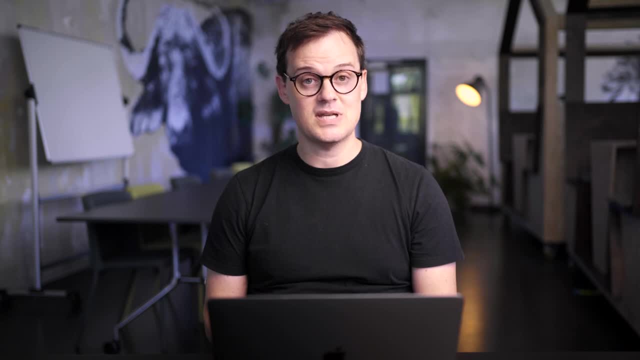 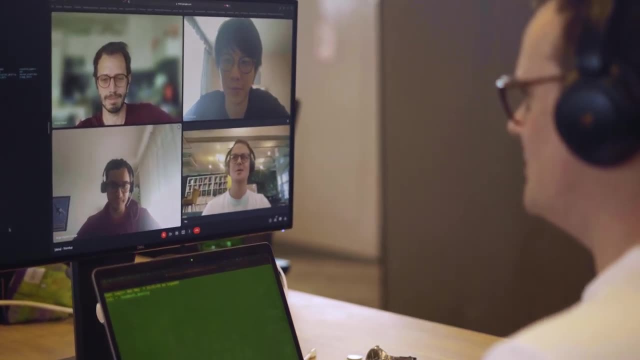 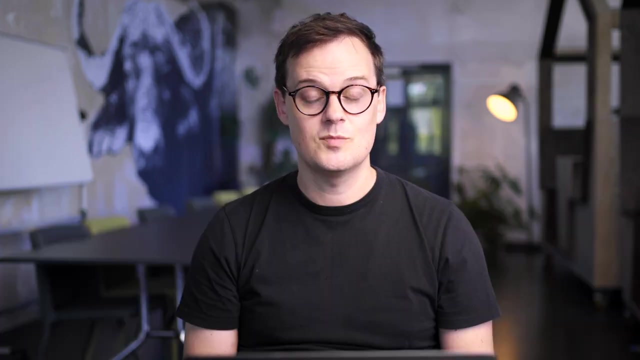 story and collaborating. Best data analysts are storytellers. They can present complex findings in a way non-data experts can understand. So do you have a knack for explaining tricky concepts in a clear and concise manner? Also, data analysts need to help the business take action derived from the data. 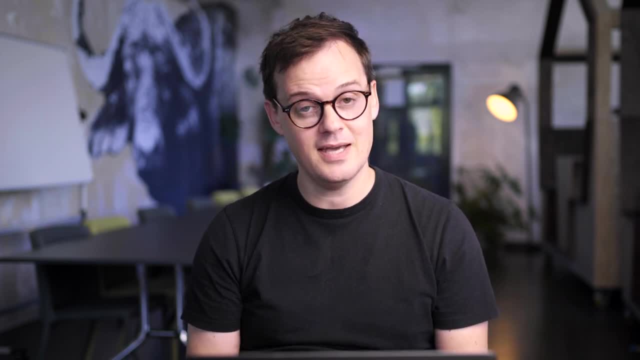 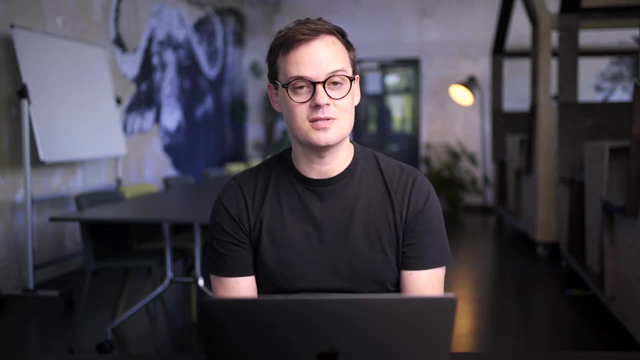 So are you a confident presenter and happy to argue your case? These qualities will serve you well in the role of data analyst. Now we've given you the questions to ask yourself. we will answer one of the questions and answer the rest of the questions in the Q&A section of the Q&A section of the Q&A section. So let's start with the first question. What is a good career move for a data analyst, And here are some reasons why: A competitive salary Based on data submitted by over 5,000 data analysts. the average base salary for a data analyst in the United States is around $75,000.. So a career as a data analyst could see you earning well above average salaries. Not only that, data analysts can expect strong salary growth as they gain more experience in the job market. A large factor in this has to do with the lack of highly experienced data analysts in the job market. 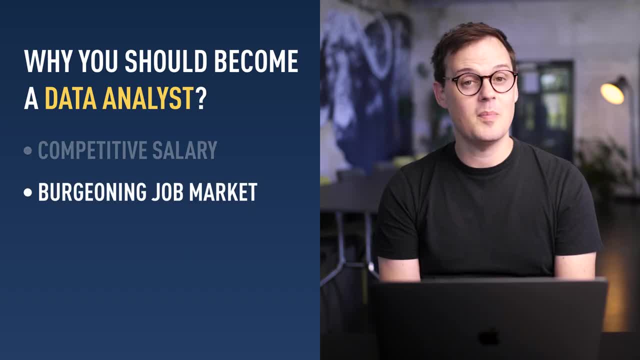 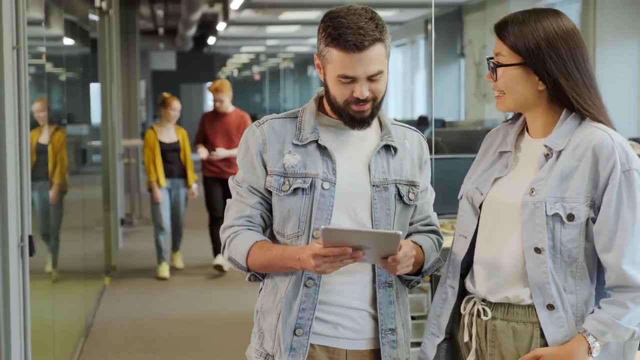 And this brings us on to the next point: a burgeoning job market. So, as we've already mentioned, there is an increasing demand for talented data analysts. More and more business sectors are transitioning towards a digital-first approach And, with the rise of connected devices and smartphone usage, 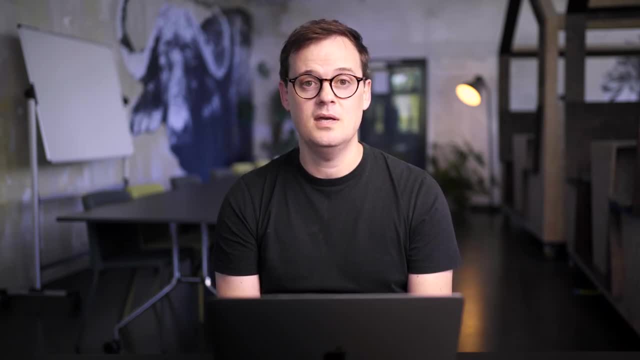 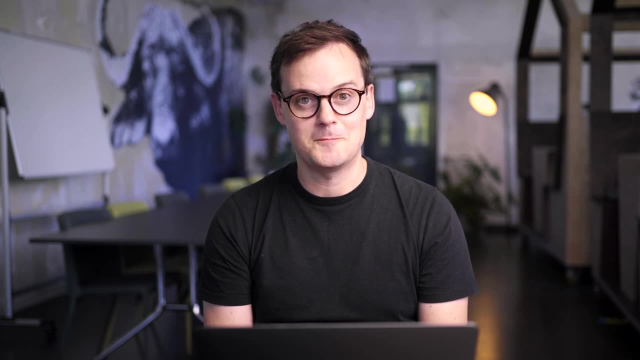 et cetera. the amount of data being generated by the modern economy is growing almost exponentially. Associated with this growth is an increasing need for data literate people in the job market. But supply is not meeting demand. Data isn't going anywhere, and neither are data analysts. 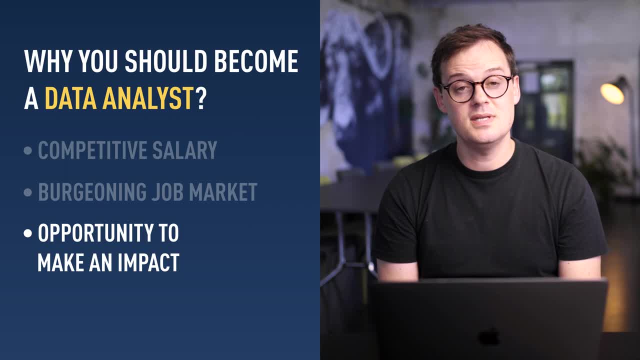 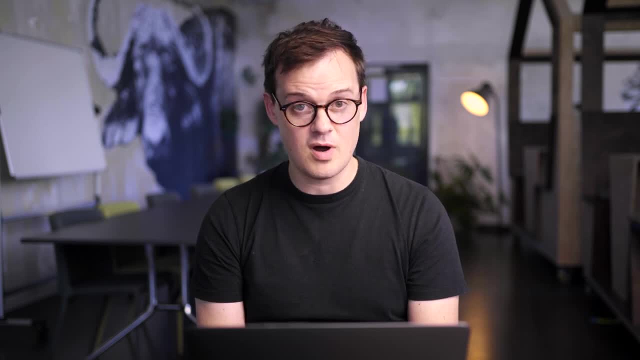 So this is an excellent job market to be a part of The opportunity to make an impact. Analytics plays a crucial role in how decisions are made. As a data analyst, you have an opportunity to drive business strategy and have a real impact on how the business moves forward. 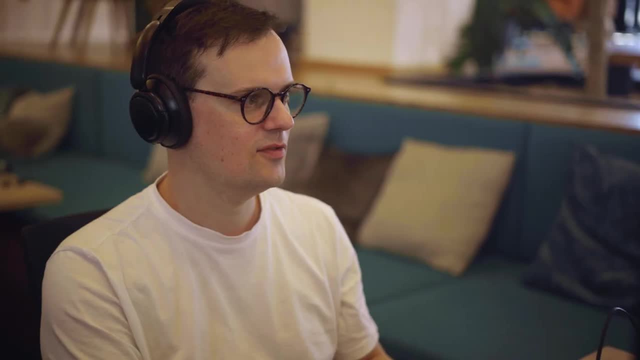 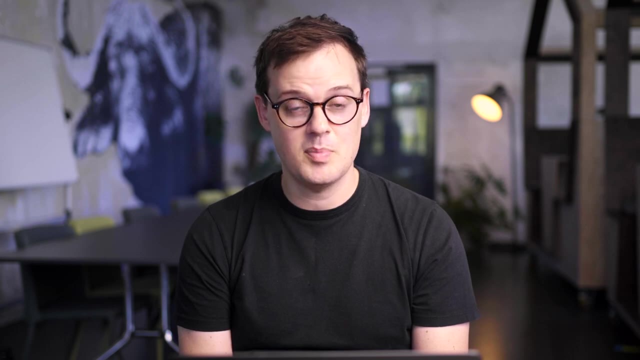 You'll get to the heart of complex business challenges, working closely with key stakeholders and using your expertise to advise on the best course of action. In this respect, you'll have a direct hand to play in the company's success and extremely rewarding. 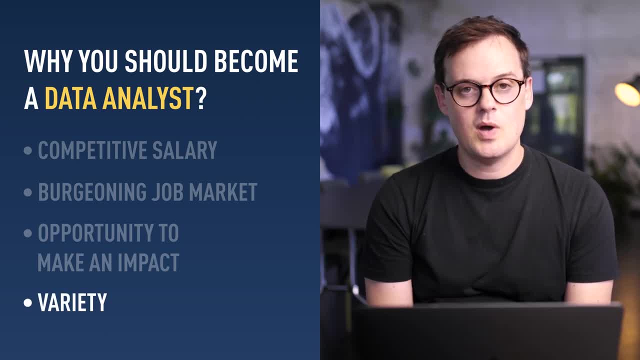 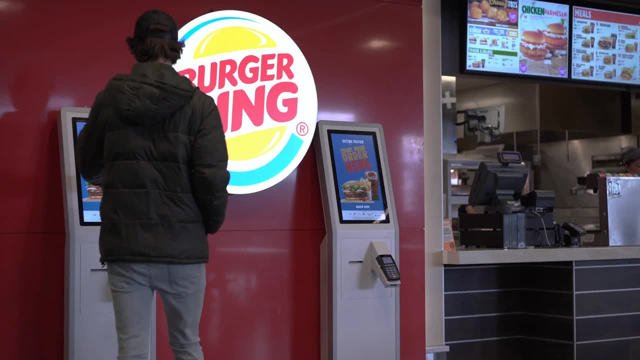 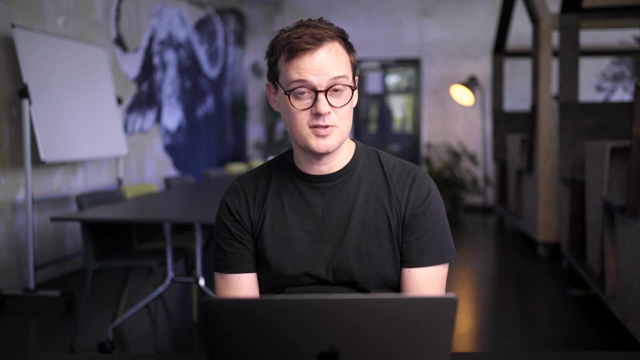 Variety. Data is absolutely everywhere, and there are opportunities for data analysts across a variety of industries and organizations. From hospitals and healthcare to fast food and fashion, from retail and marketing through insurance and technology, possibilities are endless. So if you're looking for a career that offers variety, 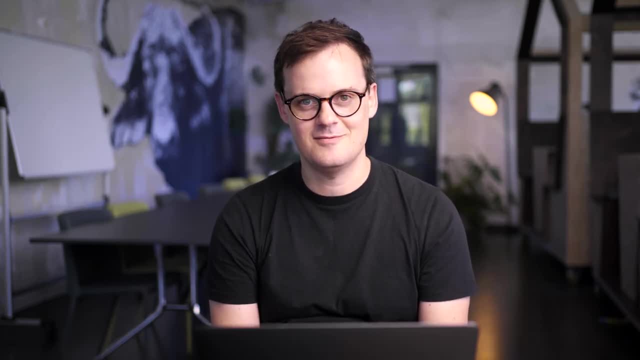 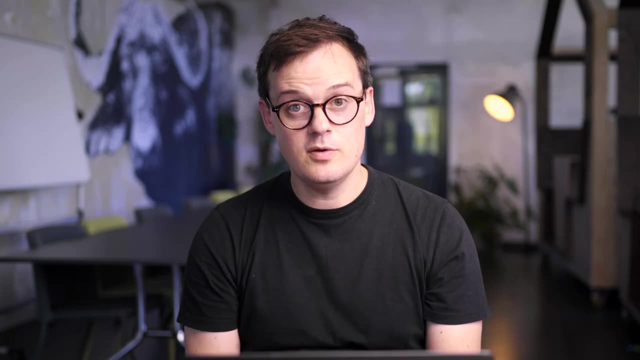 you'll certainly want to consider becoming a data analyst. Well, this is everything we've prepared for you today. Now that you know what to ask yourself, take a moment for some honesty and insight. Do note, though, these skills aren't always inherent in your career.